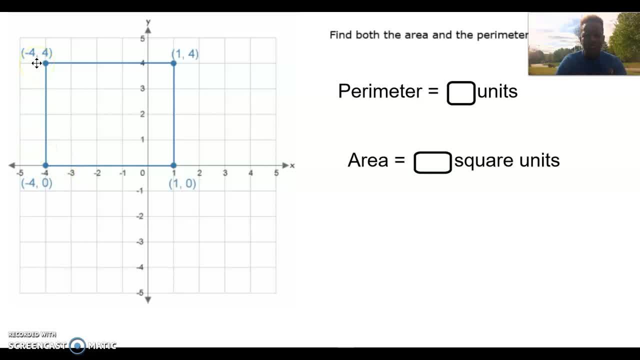 measurement All All the way around this rectangle. So what do we know about rectangles? We know that two of their sides are identical. okay, They're parallel sides, So these two will have the same length and these two will have the same length. What do we need to do? Find the length of them, So let's. 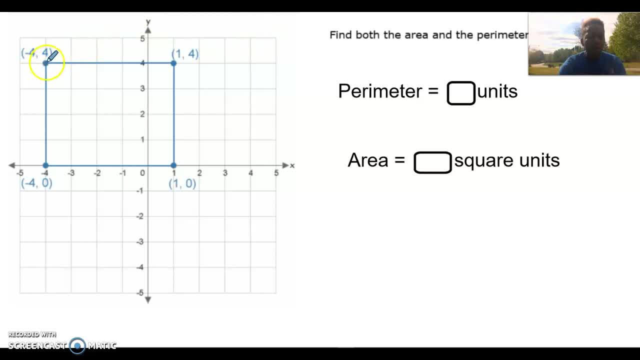 go ahead and let me show you how to do that. So I'm going to start here at my vertex. all right, So this is my zero One, two, three, four, five. So that means the length of this side right here. I'm going to try to keep it. 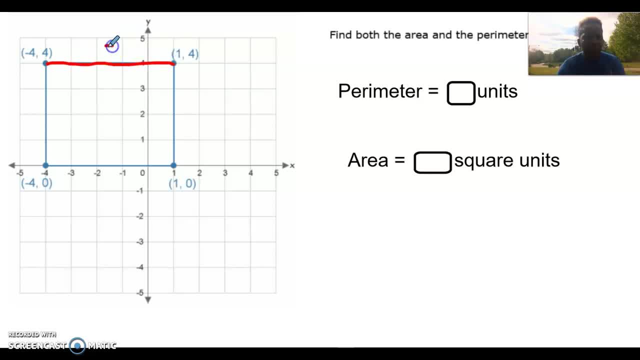 straight is five units. So that means the one down here is also what? Absolutely It's also five units. So now we need to figure out what is the measurement of our sides. the other one, OK. So what I'm going to do here is that these lines here are intersections that are 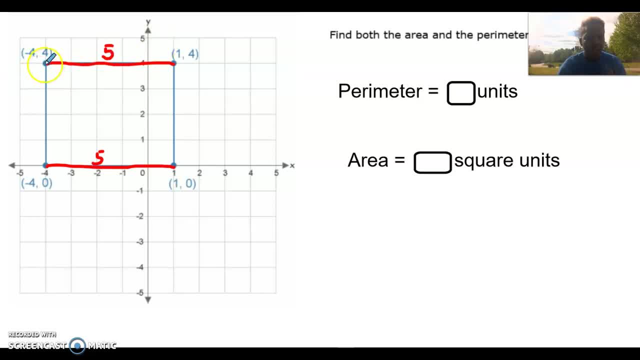 parallel. So I'm going to fill in the nine here. I'm gonna throw in the none Richtung designation because there are so many foxes on my side. all of these are oscillations that are parallel, So let me go ahead and get- let's go with green, So let's count the side- the measurement Zero. 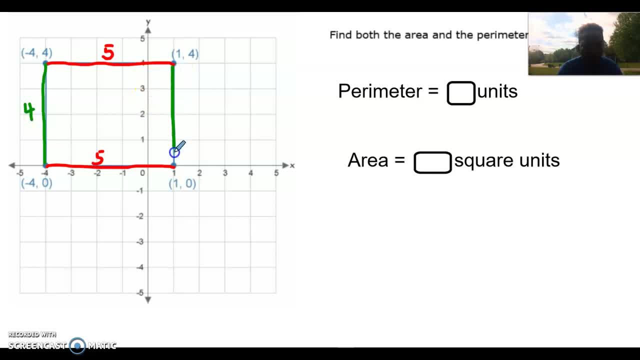 one, two, three, four. So this line segment has a measurement of four units, which means the opposite side also has a measurement of four units. units. How do we know? Because it's a rectangle, Two identical pairs. So how do we calculate the? 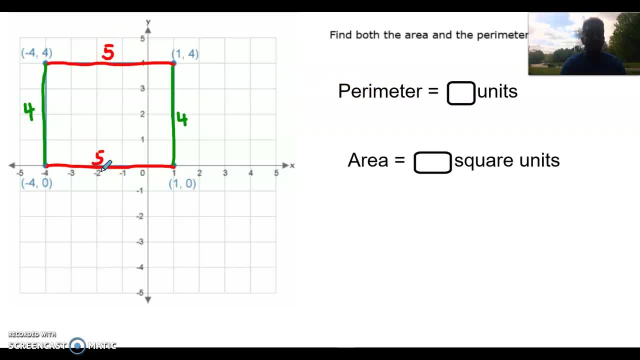 perimeter. Well, we have 5 plus 5 gives us 10. And then we have 4 plus 4 gives us 8. So 10 plus 4 is 18 units. Okay, If you need to rewind that and watch it, go ahead and do so. Okay. so now let's. 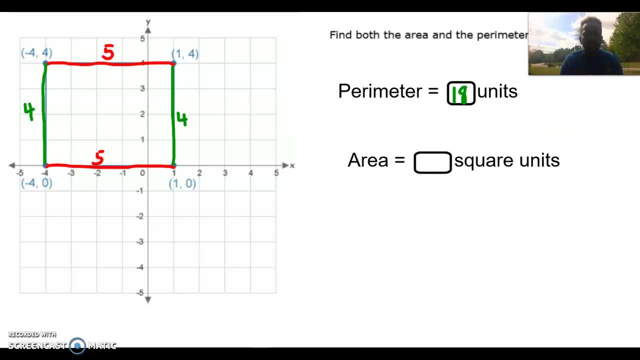 continue with finding the area. We studied area guys. What do we know about a rectangle and its area? Well, we know that we can use the formula. Does anyone remember the formula for area of a rectangle? Uh-huh, Area equals base times height. Or some will say: what about length times width?